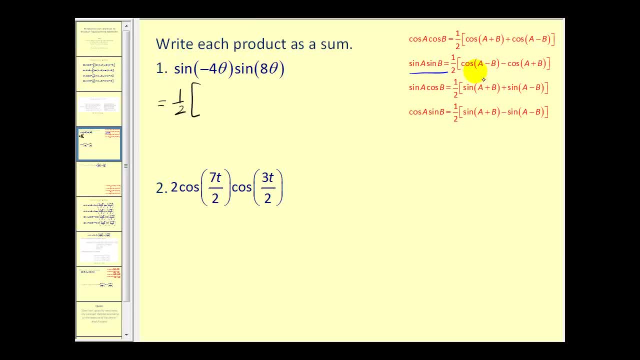 This will equal one half times the quantity cosine A minus B, So negative four theta minus eight theta minus cosine, of negative four theta plus eight theta, And that's pretty much it. We have to simplify this and we now have the product as a sum. 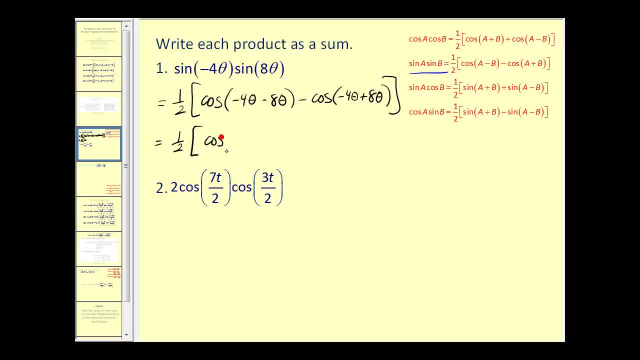 Negative four theta minus eight theta would be the cosine negative twelve theta minus cosine negative: four theta plus eight theta would be four theta. So we've taken this product and written it as a sum. Let's go ahead and try another. Here we have two times cosine, seven t over two times cosine, three t over two. 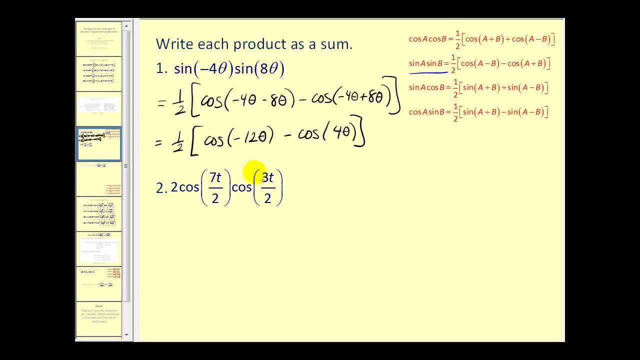 Notice, we do have a coefficient of two here, so we have to be careful with that. We have the product of two cosine functions. So now we're looking at this first identity, where angle A is seven t over two And angle B is three t over two. 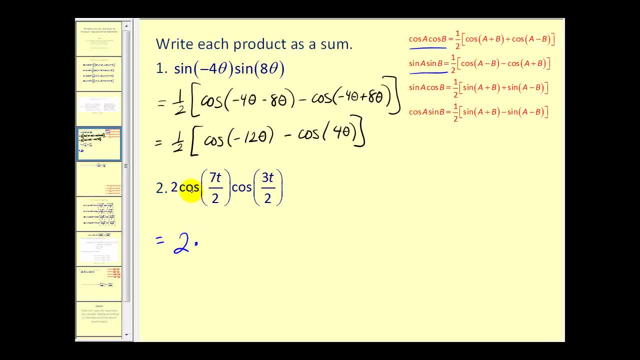 So this will equal two times, one half times, the quantity cosine of A plus B plus cosine A minus B. So be careful. We did have a coefficient of two. These simplify out And we're left with cosine of. this would be ten t over two or five t. 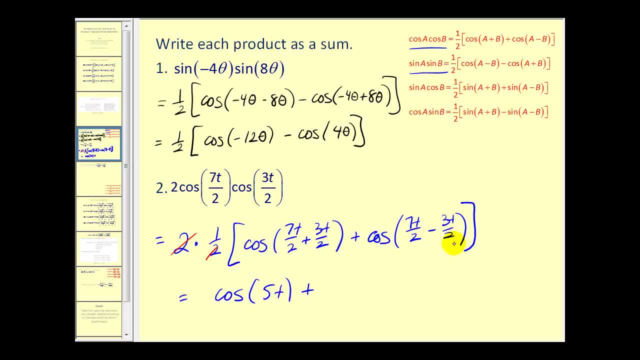 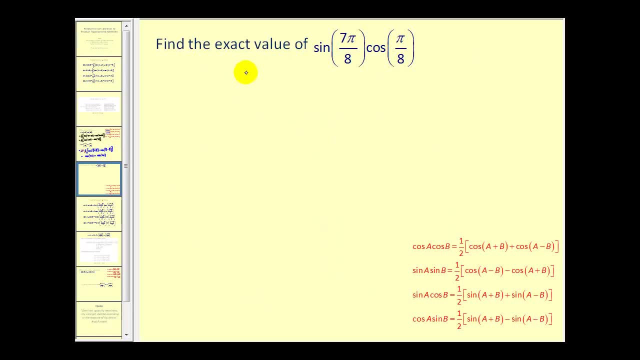 And seven t over two minus three t over two would be four t over two or just two t. Again, we've rewritten this product as a sum. Here's another type of problem. We want to find the exact value of sine A times cosine B. 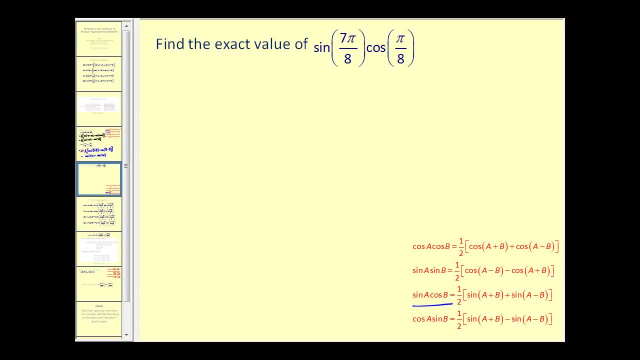 So we're looking at this identity. now Let's see how this works out: One half times the quantity of sine A plus B plus sine of the difference. So we're going to have one half and the sine of this would be eight, pi over eight, or pi. 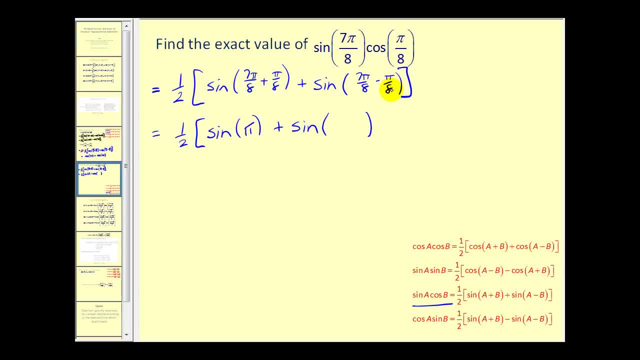 Here we're going to have seven pi over eight minus one pi over eight. That would be six pi over eight or three pi over four. So now we need to find these function values, So the sine of pi on the unit circle. this would be the point. 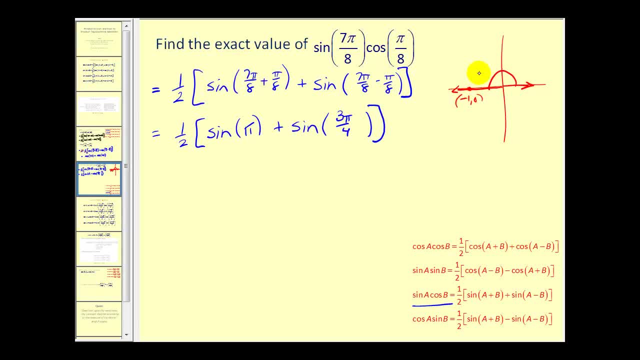 negative one, zero. Remember that sine is equal to the y-coordinate on the unit circle, So this would give us zero. Next, three pi over four would be here And our reference triangle would be a forty-five- forty-five right triangle. 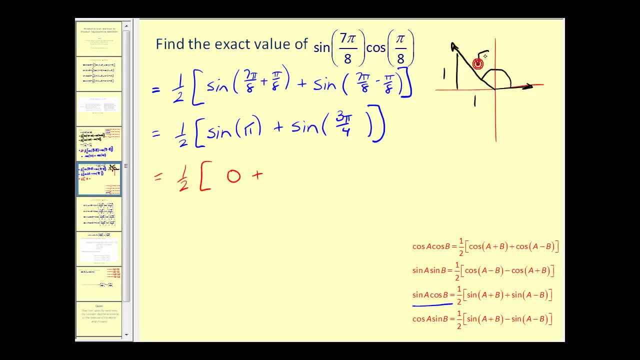 So we'd have one one square root of two. Of course this is negative. So the sine of three, pi over four, would be the opposite over a hypotenuse, one over the square root of two, which rationalizes to the square root of two over two. 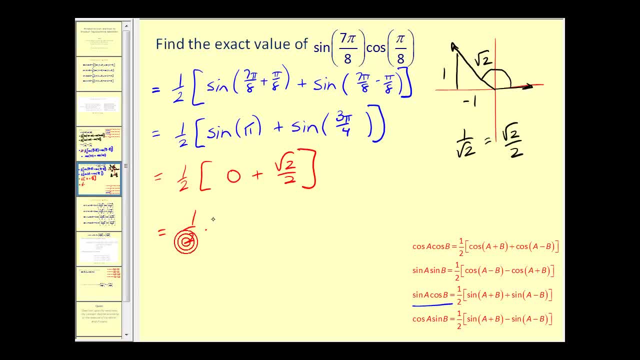 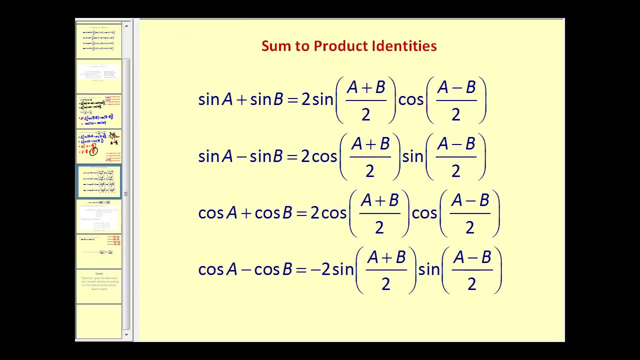 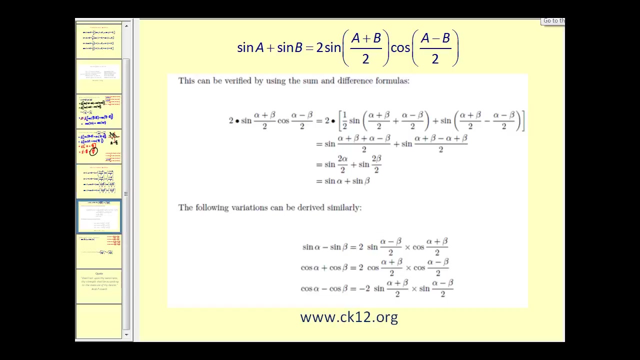 So we have one half times the square root of two over two, which equals the square root of two over four, Which is the exact value of this product. So now we have the identities that take a sum and write them as a product. I've included the derivation. 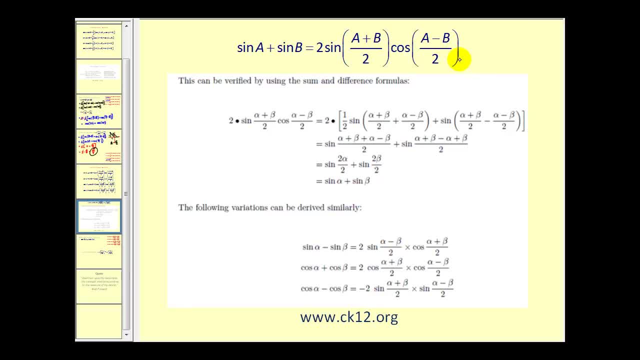 of one of them. And again, these are similar because they can be verified using the sum and difference formulas. So again, I would encourage you to pause the video and take a look at these to see where they come from. Let's go ahead and try a couple problems. 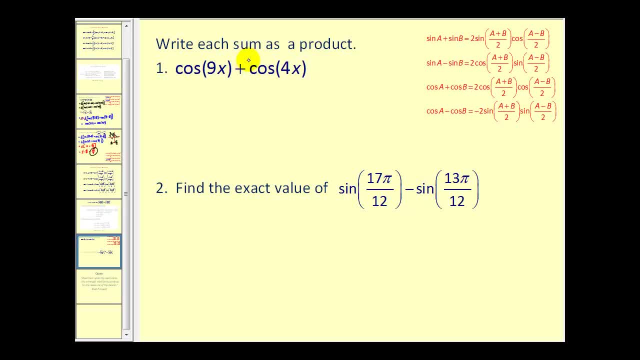 We want to write the sum now as a product. So we have the sum of cosine a plus cosine b. So we're looking at this identity here Where our angle a is nine x and our angle b is four x. So we have this will be equal to two. 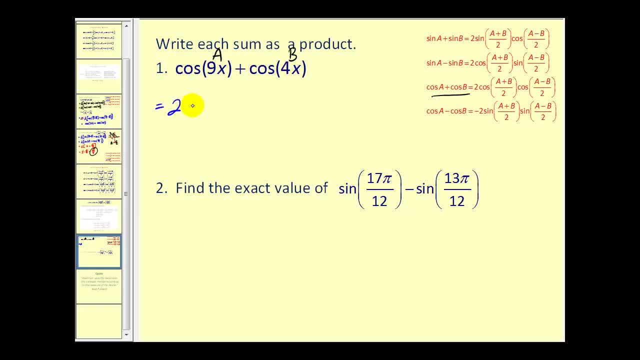 times cosine a plus b divided by two: Well, nine x plus four x is thirteen x. over two times cosine of a minus b divided by two: Well, nine x minus four x is five x. And there it is. We've rewritten this sum as a product. 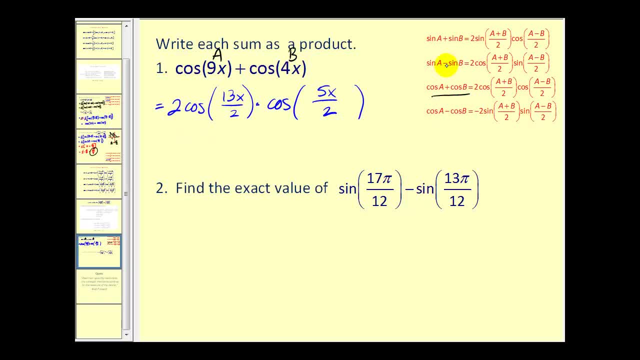 Again. once we have these identities, there's not a lot to it. Just got to be very careful with the details. Okay, on this last problem, we want to find the exact value of sine seventeen pi twelfths minus the sine of thirteen pi twelfths. 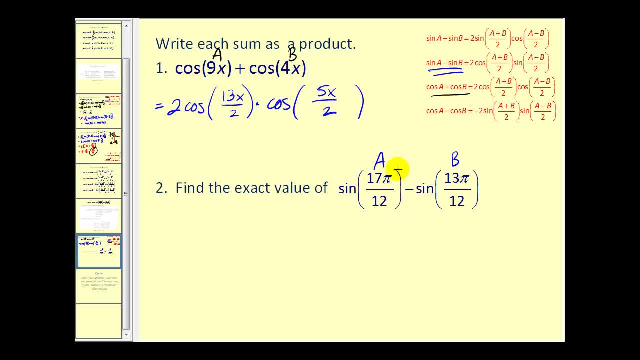 So we know that our angle a will be seventeen pi twelfths And angle b will be thirteen pi twelfths, So we'll be using this identity here. So this will be equal to two times the cosine of the sum of the angles divided by two. 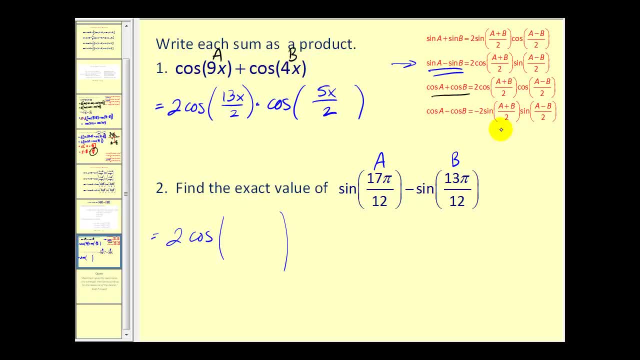 Well, the sum of these angles would be thirty pi twelfths, Which will simplify to five pi over two. So we have five pi over two divided by two, times the sine of the difference of the angles. divided by two, The difference of the angles would be: 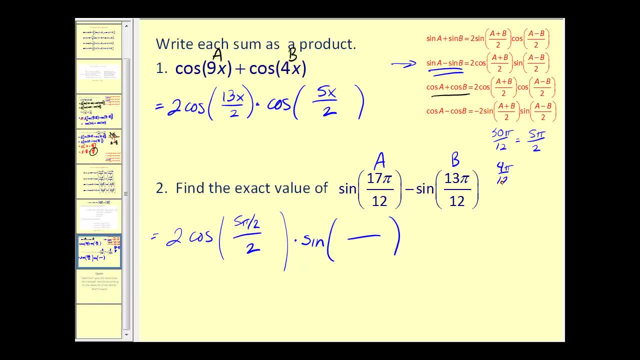 four pi twelfths, which is equal to pi over three. So we have pi over three divided by two. Let's go ahead and simplify our angles. Remember, dividing by two is the same as multiplying by one half. So this would be five pi fourths. 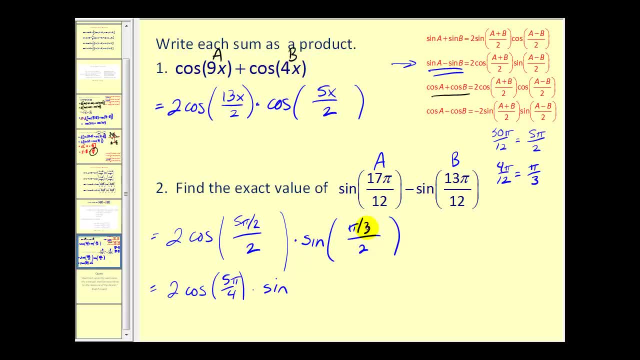 times the sine of pi over six. Okay, we need to find these function values and then find the product. So again, we don't have our unit circle handy. Let's go ahead and sketch these in standard position: Five pi over four. 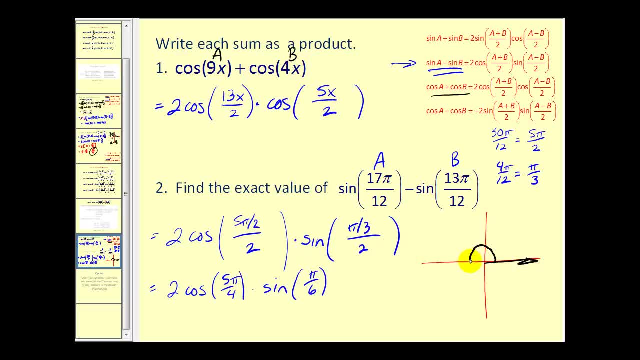 There's pi Or four fourths pi. So we need to go one fourth of a pi more. This produces a reference triangle of a forty, five, forty, five, ninety right triangle. So we have one one square root two. Of course, both the x and the y coordinates are negative. 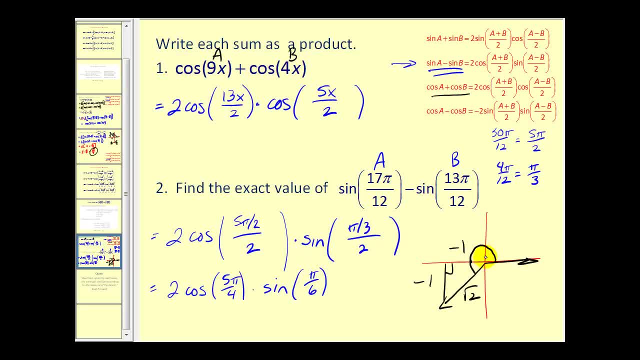 So the cosine of five pi over four would be negative. one over square root, two. Rationalized that would be negative square root, two over two. Now we need to find the sine of pi over six. Well, pi over six radians would be here With a reference triangle of a thirty, sixty, ninety.